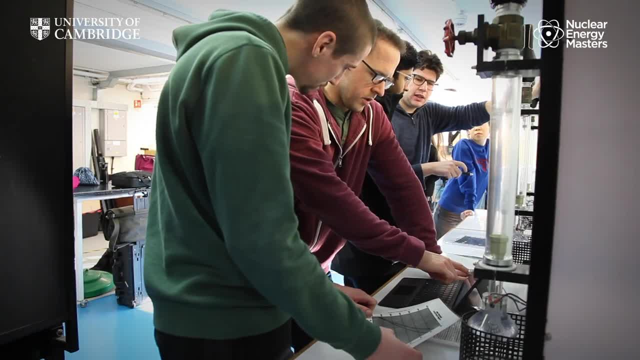 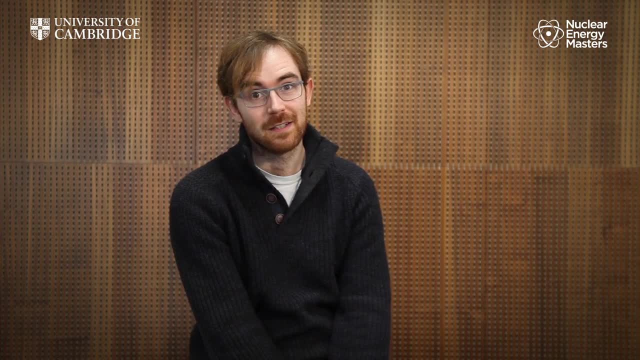 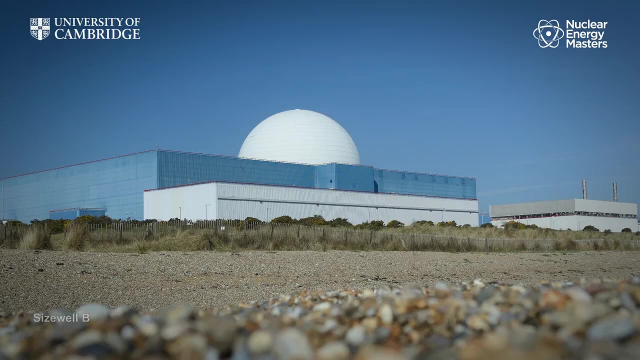 Many of our graduates have gone on to fill these roles as experts in the science and policy of nuclear energy. Destinations have ranged between research labs, international organisations, reactor design and power companies. Many students have also used nuclear energy as a springboard to careers in the wider energy sector. 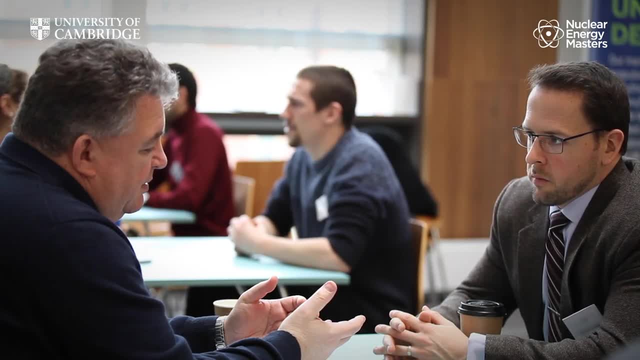 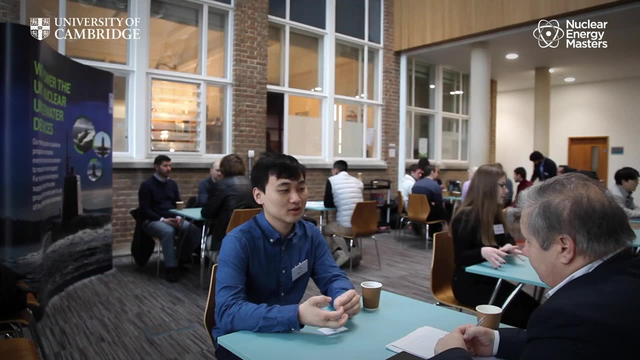 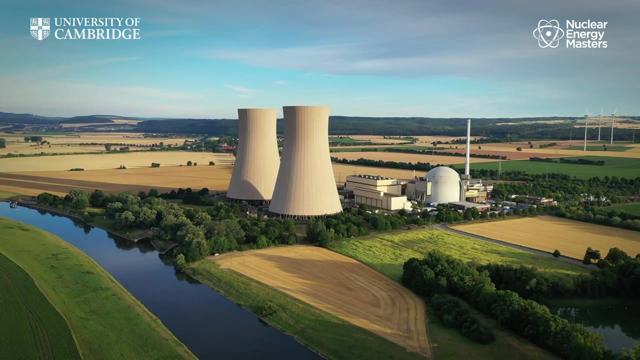 The course is supported by an industry club composed of the biggest companies on the UK nuclear scene. As well as sponsoring the course, the club proposes research projects for students, exposing them to problems relevant to industry while allowing them a fast-track interview process. Many of our alumni are now employed by industry club members. 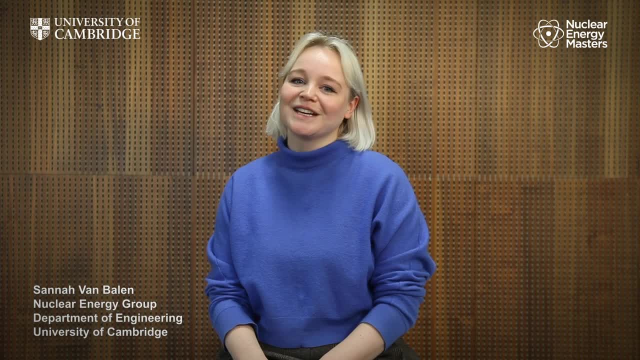 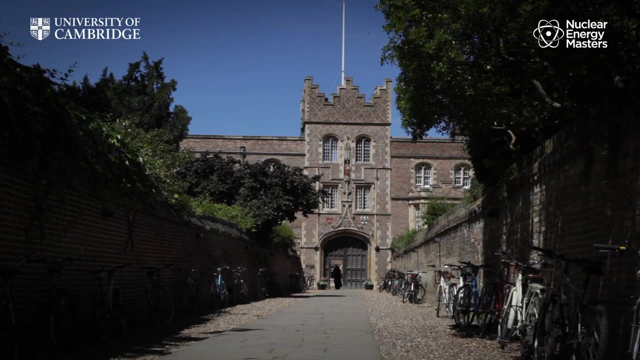 Studying nuclear energy at the University of Cambridge is truly a unique experience. You don't only join the engineering department, which is where you will spend time with your course mates, but you also join a college, And this is where you get to meet students. 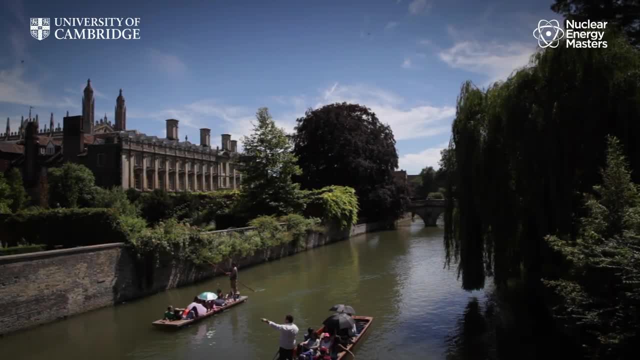 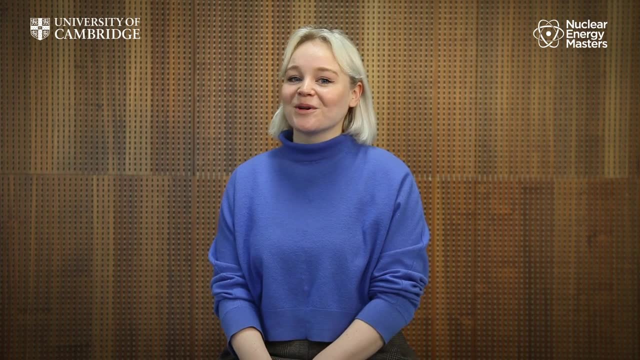 students pursuing different degrees join fun societies and participate in the typical Cambridge traditions. As an alumna from the MPhil in Nuclear Energy, I can tell you that one of the most memorable aspects of the course are the visits to nuclear sites. In my year we visited the Column Centre. 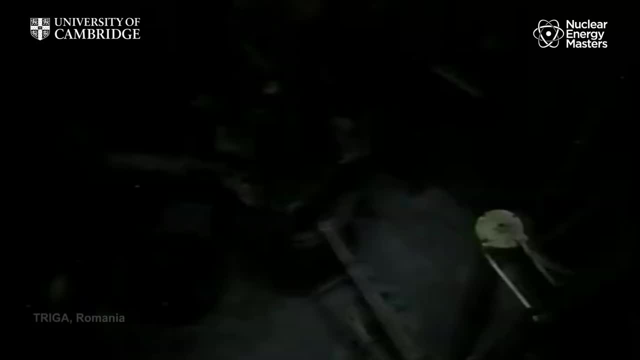 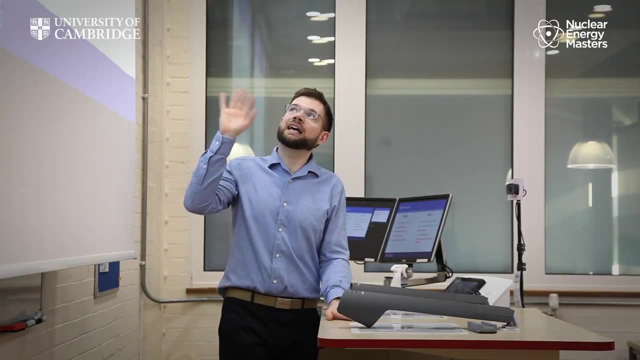 for Fusion Energy and Sizewell B in the UK, as well as the Triga test reactor in Romania. Alongside the research projects, these experiences help connect what you learn in the lectures and seminars To real-life applications of nuclear technology. 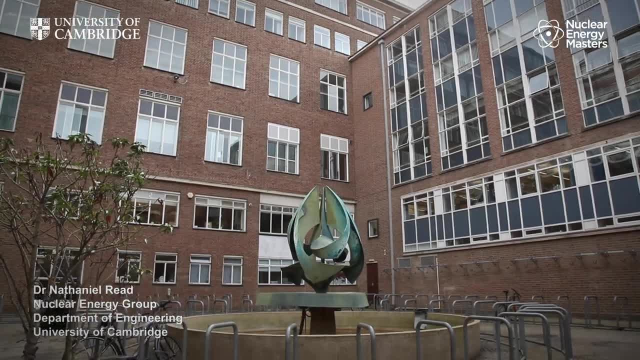 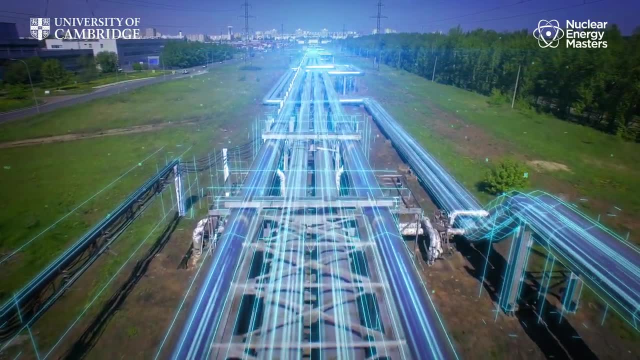 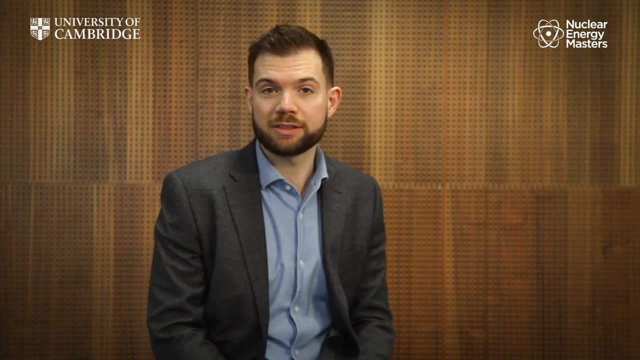 The Nuclear Energy Masters course is based mainly here at the Department of Engineering. However, nuclear energy calls for a wide variety of knowledge and skills. Our course is highly relevant to the 21st century's energy needs. The world needs not only nuclear engineers, but experts in energy policy management and economics. Our curriculum 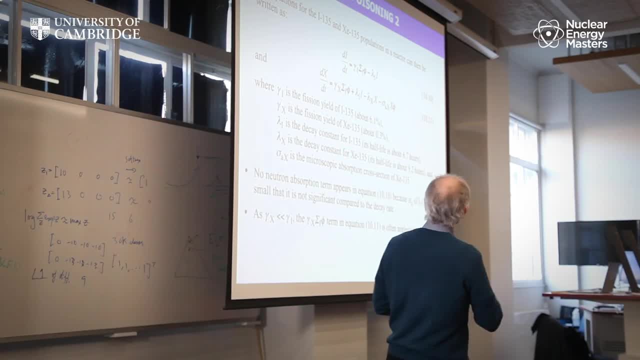 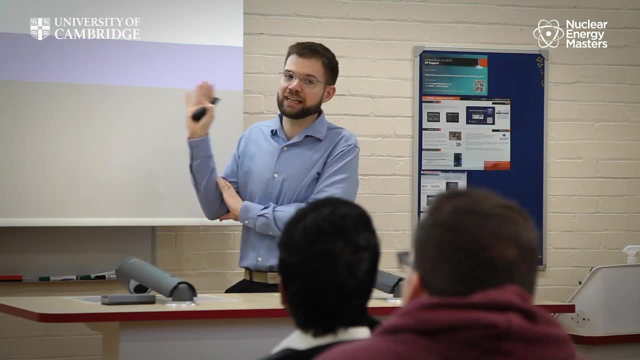 is therefore highly flexible. Students can choose to focus entirely on nuclear engineering, taking modules specifically for nuclear engineering, Or students can choose to take between one and five of their ten modules from partners in the departments of Engineering, Chemical Engineering, Physics and the Judge Business. 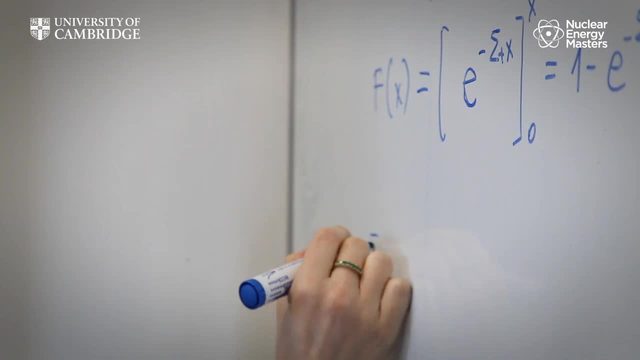 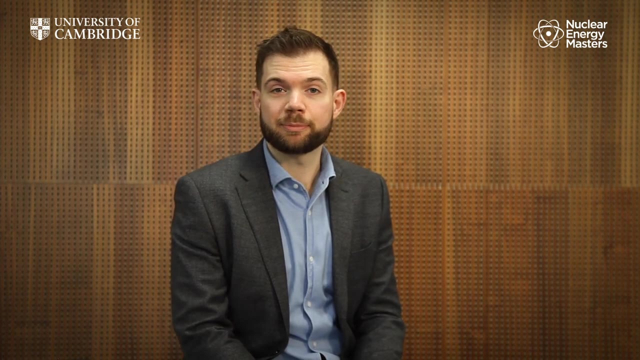 School. We pride ourselves on excellence in teaching, with a significant amount of contact with teaching staff In the first two terms. as well as lectures, students can expect small group tutorials, detailed feedback on their performance and mentoring Over the summer students will.